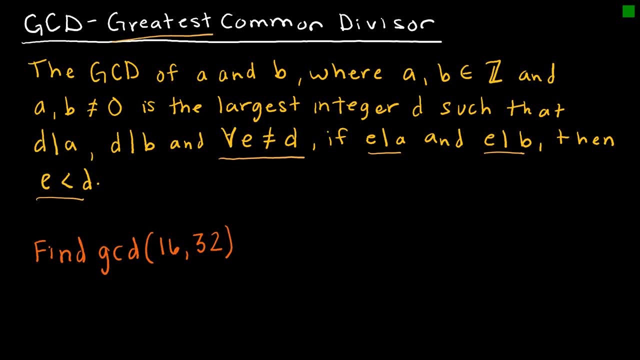 greatest part of it. So it's the highest number, Highest value, integer value that divides both A and B. So pretty straightforward Again. I'm sure that we've all done these before. What I want to do is look at a few different ways that. 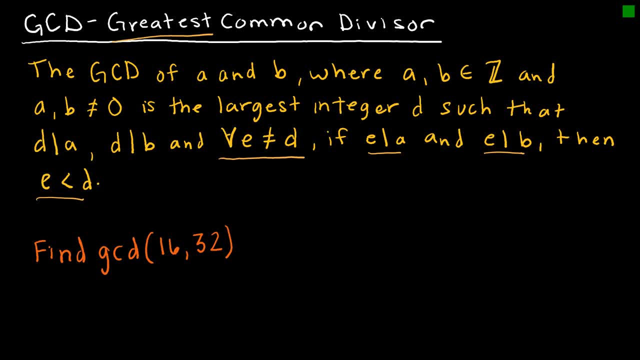 you can go about finding the GCD. So, and these are all again very elementary, So if I was looking at 16, I would say 16, the divisors are one, because one goes into 16, two. 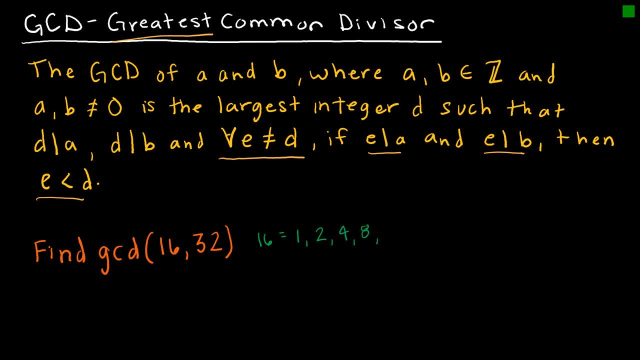 four goes into 16,, eight goes into 16, and 16 goes in a 16.. And then I could do the same for 32.. So one and two, and four and eight, And again we're just looking for the one that that matches basically. 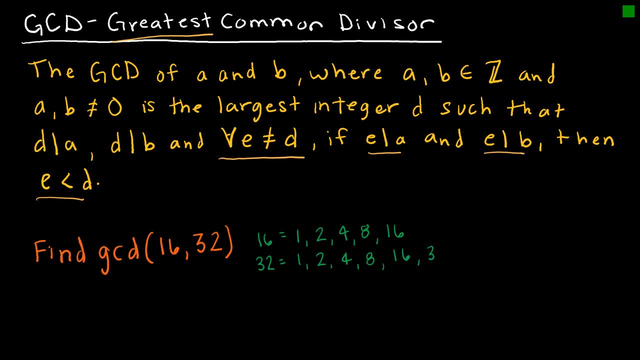 matches up and 16, and 32.. And so, again, all I'm looking for is what is the highest number that appears in both of those lists, are the both of those lists, and that number is 16.. So, again, I don't have to explain to you how to find a GCD, I'm sure 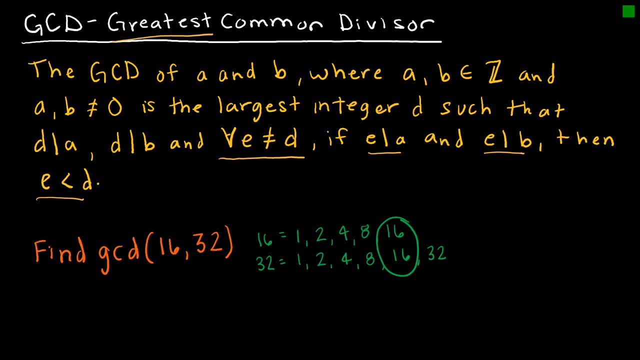 you've done it several times, But now let's take a look at how I could do this using prime numbers, because obviously we're dealing with primes right now. So I could look at 16 and look at the prime factorization And the GCD or, I'm sorry, the prime factorization of 16, again, I could make. 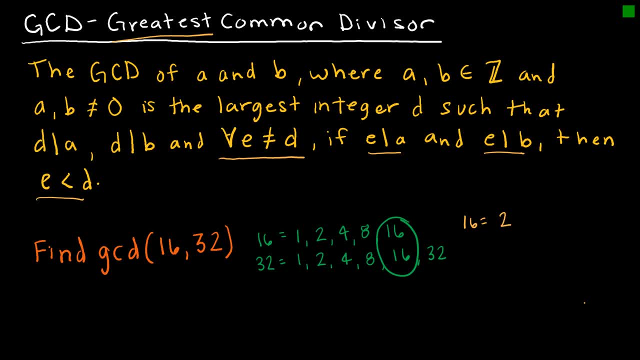 a tree if I needed to. But really I'm just saying it's 2 times 2 times 2 times 2, or 2 to the fourth, And then if I write 32 as the prime factorization, it's 2 to the fifth, And if I'm 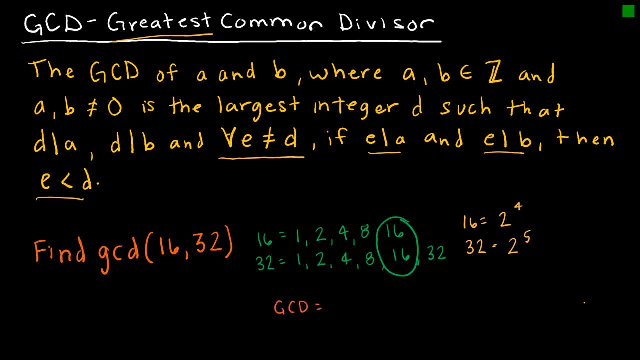 looking at the GCD, I'm looking at the most number of times that a prime occurs in common with one another. So here's 2 to the fourth, this is 2 to the fifth and this is 2 to the fifth. 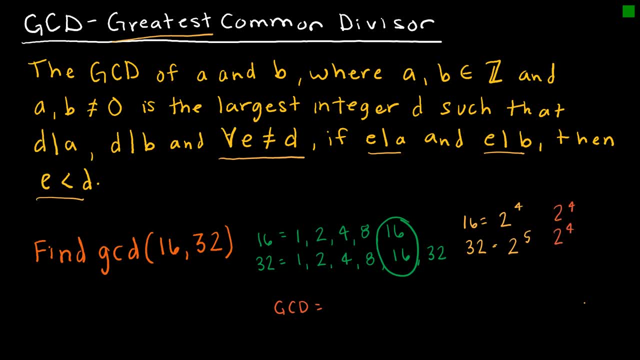 the fifth, So two to the fourth, and this is like two to the fourth times two, So two to the fourth is the greatest number of times that occurs in both, And so that is the greatest common divisor, which is, of course, 16.. So the answer is 16, either way you look at it, But obviously 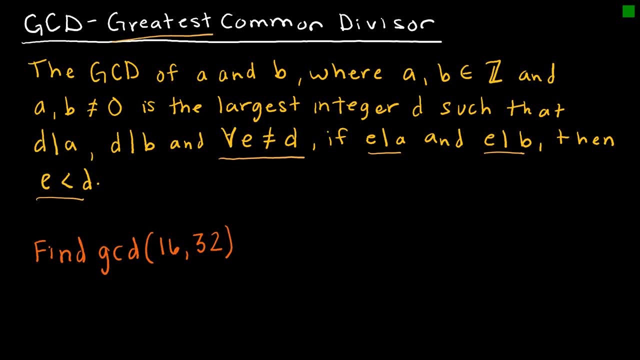 greatest part of it. So it's the highest number, Highest value, integer value that divides both A and B. So pretty straightforward Again. I'm sure that we've all done these before. What I want to do is look at a few different ways that. 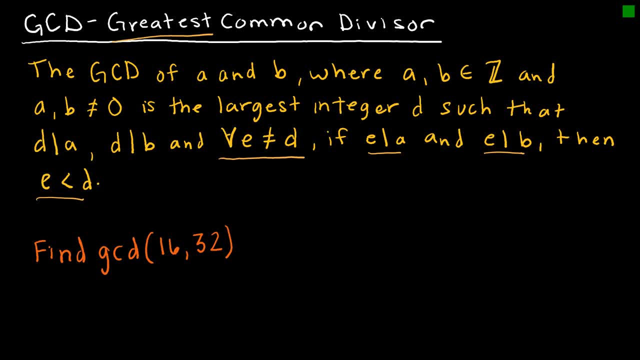 you can go about finding the GCD. So, and these are all again very elementary, So if I was looking at 16, I would say 16, the divisors are one, because one goes into 16, two. 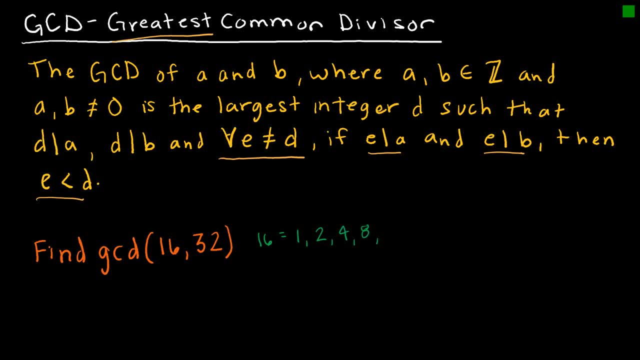 four goes into 16,, eight goes into 16, and 16 goes into 16.. And then I could do the same for 32.. So one and two, and four and eight, And again we're just looking for the one that matches. 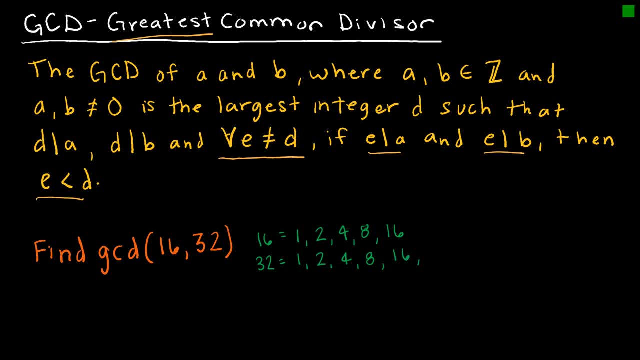 basically matches up And 16 and 32.. And so, again, all I'm looking for is what is the highest number that appears in both of those lists, And that number is 16.. So, again, I don't have to explain to you how to find a GCD, I'm sure you've. 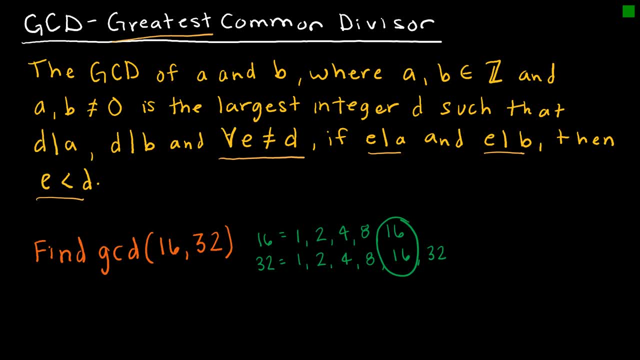 done it several times, But now let's take a look at how I could do this using prime numbers, because obviously we're dealing with primes right now, So I could look at 16. And look at the prime factorization And the GCD or, I'm sorry, the prime factorization of 16. Again, 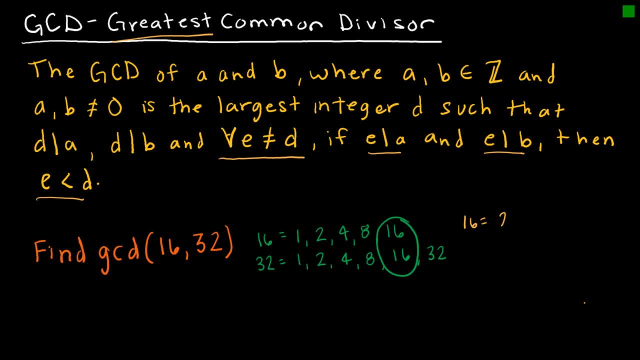 I could make a tree if I needed to, But really I'm just saying it's two times two times two times, or two to the fourth, And then if I write 32 as the prime factorization, it's two to the fifth. 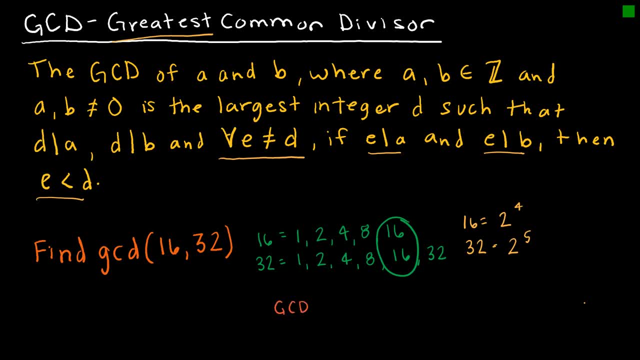 And if I'm looking at the GCD, I'm looking at the most number of times that a prime occurs in common with one another. So here's two to the fourth, this is two to the fifth, So two to the fourth, and this is like two to the fourth times two. 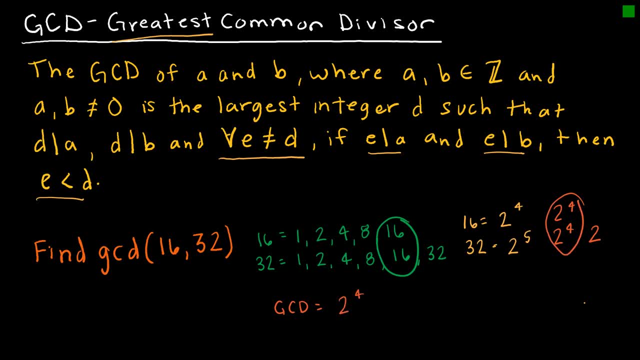 fourth is the greatest number of times that occurs in both, and so that is the greatest common divisor, which is, of course, 16. so the answer is 16 either way you look at it, but obviously looking at primes is going to be it sort of an easy. 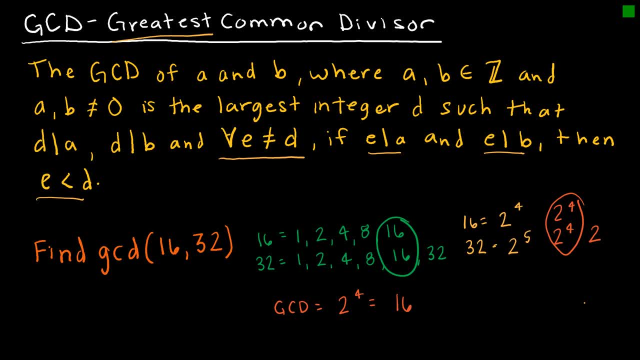 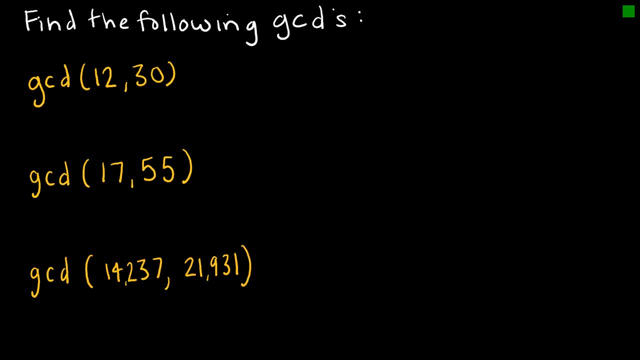 looking at primes is going to be sort of an easy way to go forward, since we're studying primes right now, So let's just do a little bit of practice. First one is 12 and 30. And again I can look at 12 and say what's the prime factorization? And 12 is two squared times three. 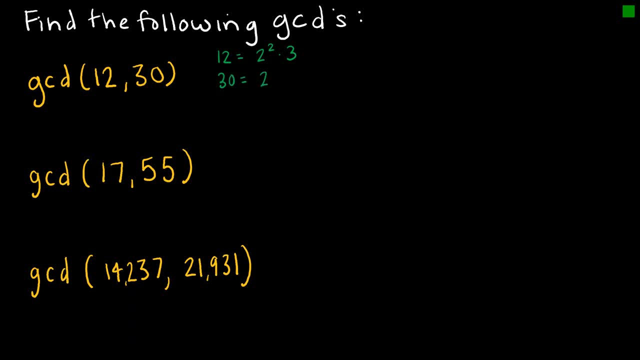 I can look at 30 and say two goes into it once. that gives me 15.. 15 is three times five, And so my GCD would be the most number of times two occurs in common, which is just once. The most number of times three occurs in common, which is just once. 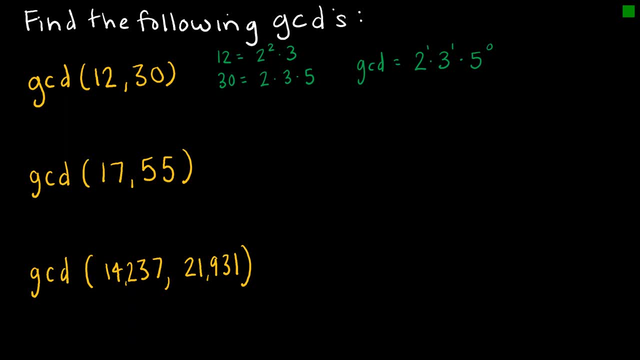 And the number of times five occurs in common, which is it doesn't five to the zero, And so my greatest common divisor here would be two times three, which is six. Again, you might be able to just figure that out very easily by looking at 12 and 30.. And that's great. I'm just showing you how. 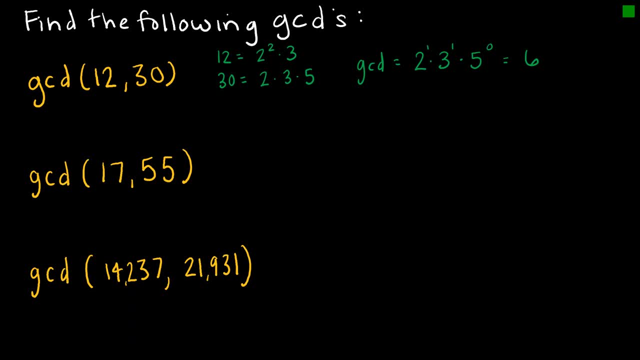 we would do it as we. as it pertains to primes. Same thing for 17.. 55.. 17 is a prime, so it's just 17.. 55, it's five times 11.. Those are both primes. So what is the greatest common divisor? It would just be one. One is the largest number. that goes. 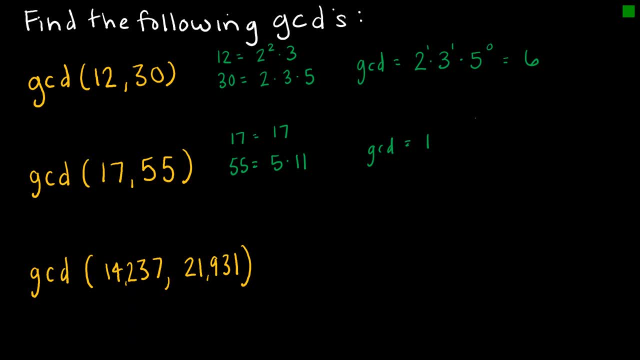 into both of those, And what I want to point out on this one is that this is considered relatively prime. So relatively prime means that they don't have any factors in common. So GCD of one. And then let's look at that last one. I don't know about you, but that just seems like something I 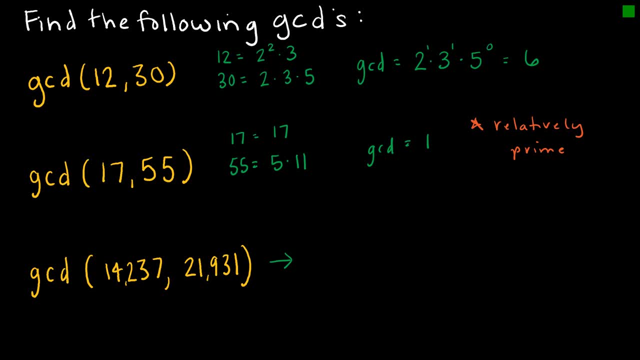 don't want to tackle, And so the reason I put it on here is to let you know there is a way to go about this, And it is Euclid's algorithm, which we'll study in a little bit, But for now I'm not. 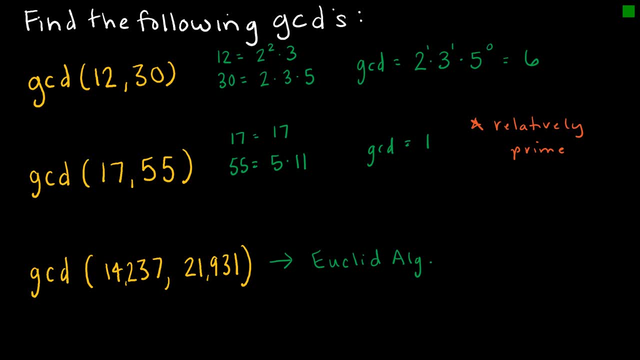 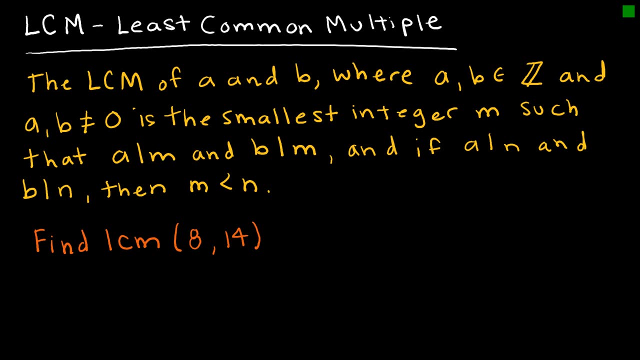 even going to try, It's just I'm going to try to find the greatest common divisor of those two values. So now let's look at the least common multiple. The least common multiple of A and B, where A and B are both integers and not equal to zero, is the smallest integer that essentially divides that. they both divide, So A divides. 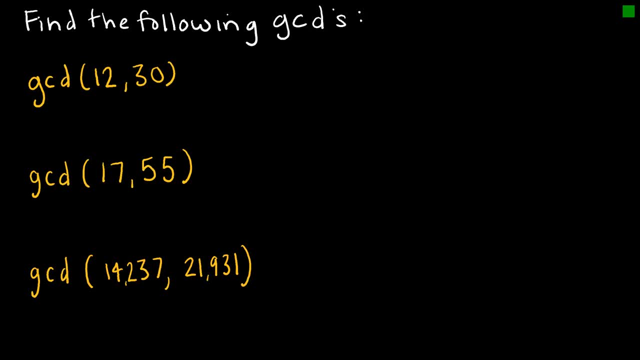 way to go forward, since we're studying primes right now, so let's just do a little bit of practice. the first one is 12 and 30, and again I can look at 12 and say what's the prime factorization. and 12 is 2 squared times 3. I can look at 30. 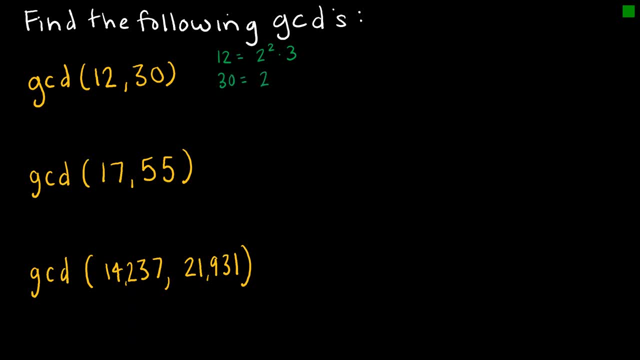 and say 2 goes into it once. that gives me 15. 15 is 3 times 5, and so my GCD would be: the most number of times 2 occurs in common, which is just once. the most number of times 3 occurs in common, which is just once. and the number of 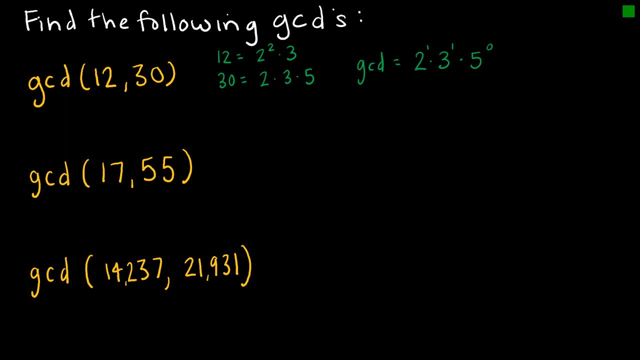 times 5 occurs in common, which is- it doesn't you 5 to the 0, and so my greatest common divisor here would be 2 times 3, which is 6. again, you might be able to just figure that out very easily by looking at 12. 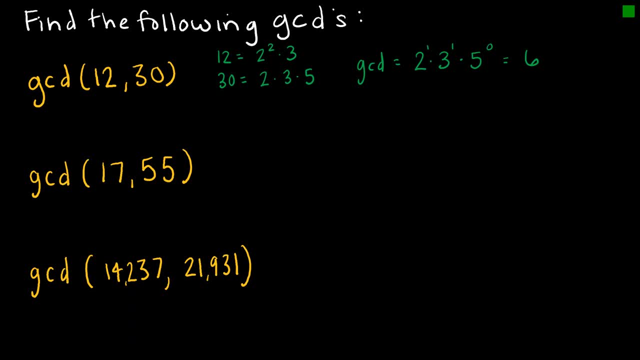 and 30, and that's great. I'm just showing you how we would do it as we. as it pertains to primes, same thing for 17 and 55. 17 is a prime, so it's just 17, 55 it's 5 times 11. 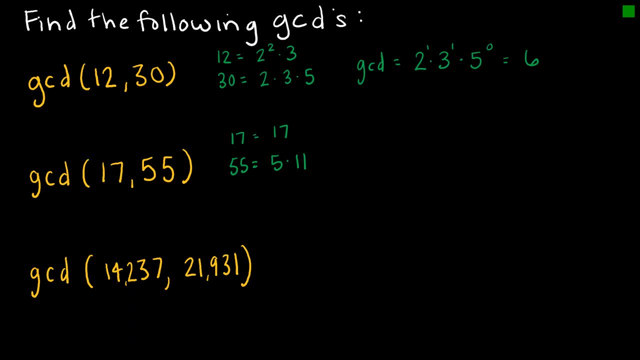 those are both primes. so what is the greatest common divisor? it would just be 1. 1 is the largest number. that goes into both of those, and what I want to point out on this one is that this is considered relatively prime. so relatively prime means that they don't have any factors in common. so the GCD of 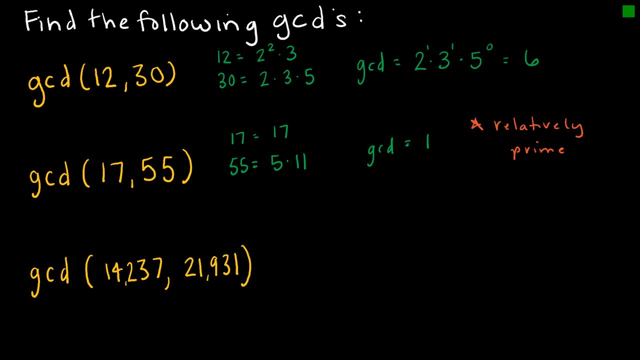 1. and then let's look at that last one. I'm going to go ahead and do a little bit of a guess and I'll just say C or generalized outcome and theнимed into a similar wrapper, I want to call it a tetrahedral. in season, the theme in 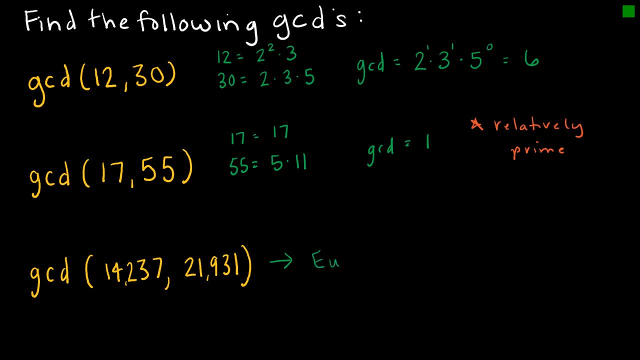 season terms. so it's a particular type of such some of the phase variable is E, E which is mixed in going to be magnesium. so E minus 1, leftover of E, S and Thereforeiration gets. I need to divide that into one plus 1. that goes. 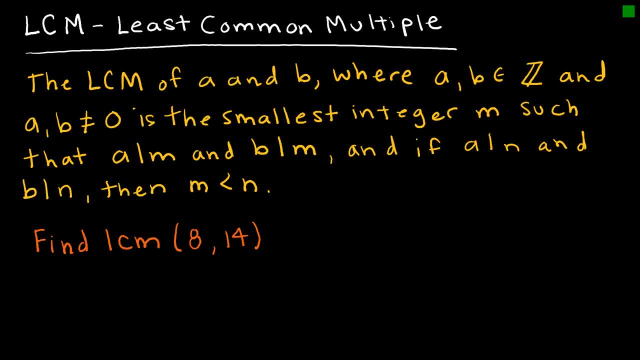 into T 1 minus materials, КонYes, and it has to be the least common multiple. well, the least common multiple I'm going to find- I have to figure out if you'd like me making something like this- and b, where a and b are both integers and not equal to zero, is the smallest integer that 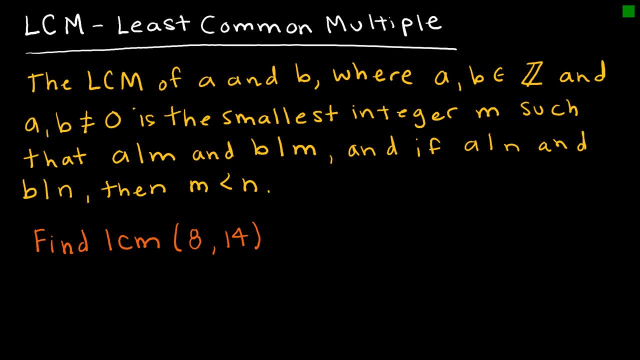 essentially divides, that they both divide. So a divides m and b divides m, And if there happens to be another integer that a divides and b divides, then m is the smallest of those, So it's the least common multiple. So again for this one, instead of looking at numbers that multiply into 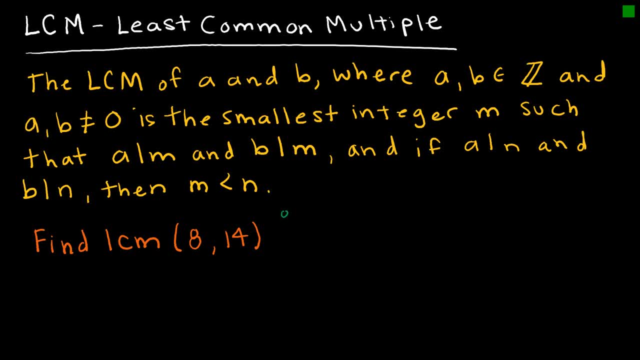 eight factors of eight. I would be looking at eight as 8,, 16,, 24,, 32,, 40,, 48,, 56,, etc. And 14 would be 14 times 1, 14 times 2,, 14 times 3.. And I could look at 8 as 8,, 16,, 24,, 32,, 40,, 48,, 56,, etc. And 14 would be 14 times 1,, 14 times 2,, 14 times 3.. 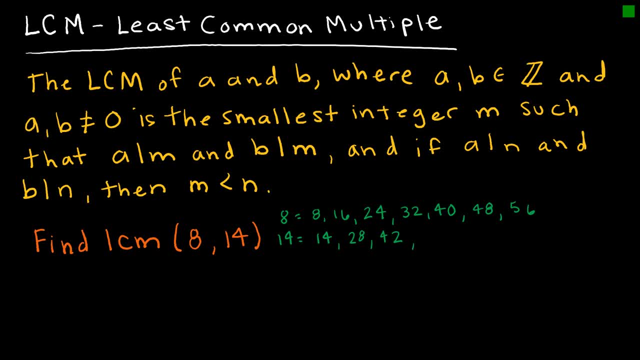 You can see, I don't have one in common yet, And so this is where it's not so fun, because then you just have to basically keep going until you find one, And so in this case, I have found that 56 would be the least common multiple. So is there a way to use primes to do this, as we did when we 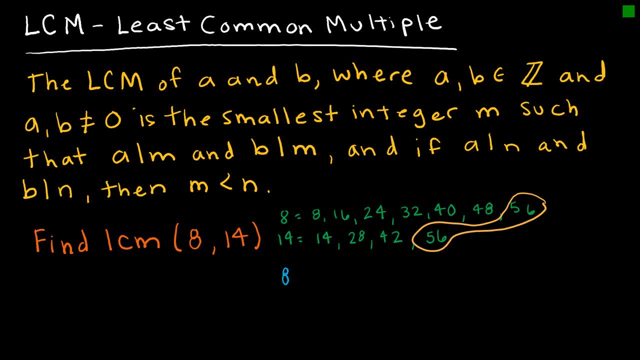 looked at the greatest common divisor. Well, let's take a look at 8.. 8 is 2 times 2 times 2.. And 14 prime factorization 2 times 7.. And so in our last example, when we were looking at the greatest, 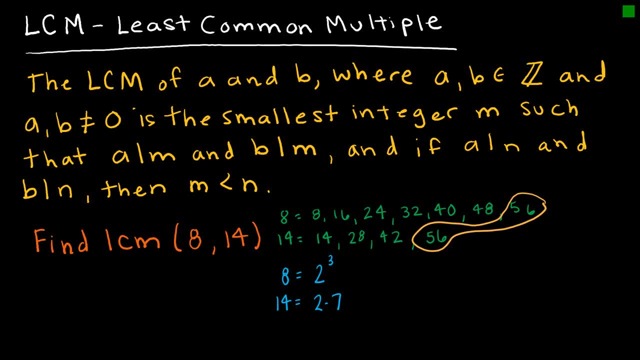 common divisor, we said how many do they have in common? And when we look at the least common multiple, we're looking at how many is the most number of times it occurs. So they have both have a 2.. What's the most number of times it occurs? 3 times. Only one of them has a 7, and it occurs. 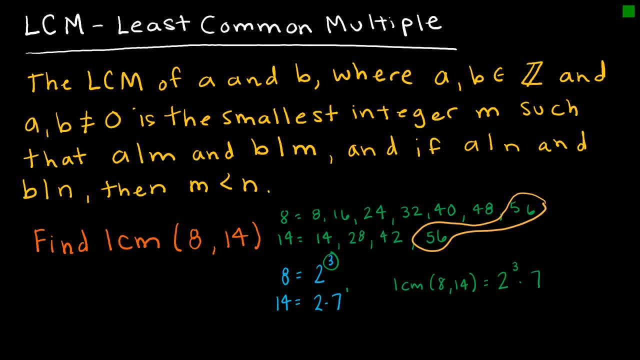 one time. So the most number of times it occurs is 3 times. So the most number of times it occurs is once. so 7 to the first. So then I'm just taking 2 to the third times 7, which is 56. So again, 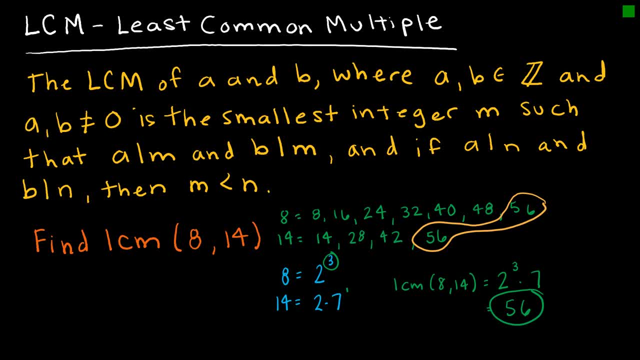 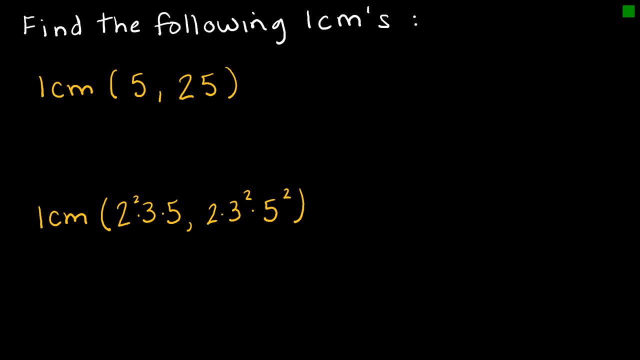 this is a strategy for us to use, especially if we already have it written as a prime factorization. So again, just a couple of practice, pretty straightforward. One thing that you can do right away- which is why I included this example- is you can say: does 5 go into 25?? 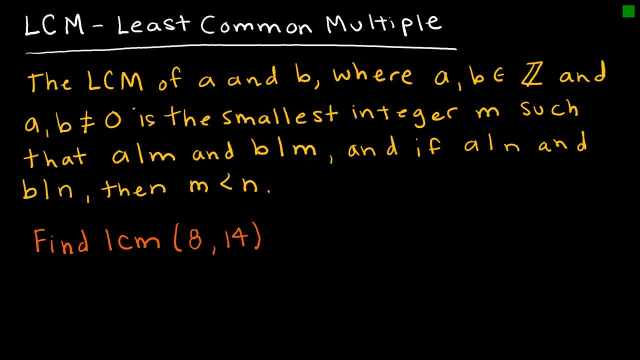 M and B divides M, And if there happens to be another integer that A divides and B divides, then M is the smallest of those, So it's the least common multiple. So again for this one, instead of looking at numbers that multiply. 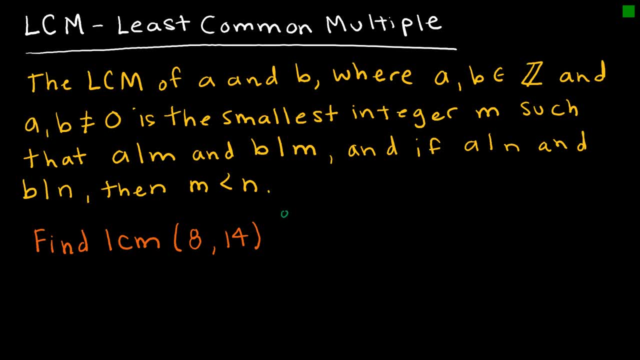 into 8, factors of 8, I would be looking at 8 as 8,, 16,, 24,, 32,, 40,, 48,, 56, etc. And 14 would be 14 times 1,, 14 times 2,, 14 times 3.. And I can see I don't have one in common yet, And so 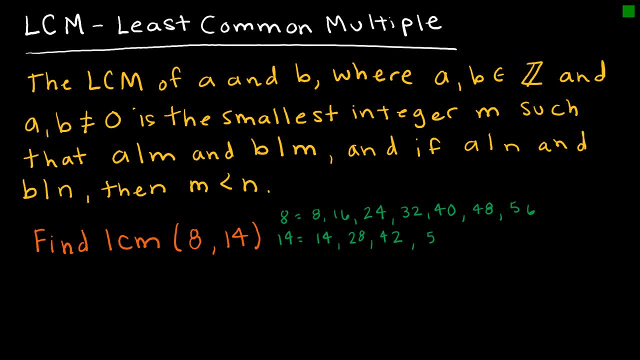 this is where it's not so fun, because then you just have to basically keep going until you find one, And so in this case, I have found that 56 would be the least common multiple. So is there a way to use primes to do this, as we did when we looked at the greatest common divisor? 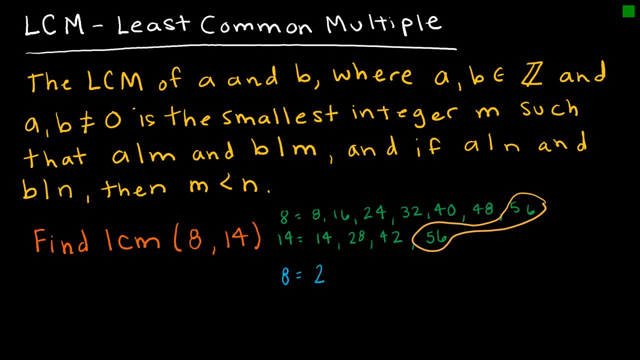 Well, let's take a look at 8.. 8 is 2 times 2 times 2. And 14, prime factorization, 2 times 7.. And so in our last example, when we were looking at the greatest common divisor, 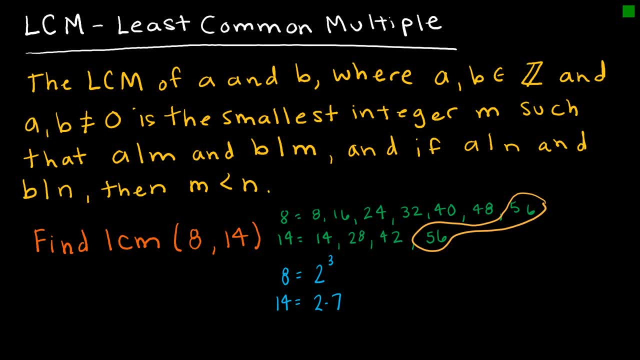 we said how many do they have in common? And when we look at the least common multiple, we're looking at how many is the most number of times it occurs. So they have a 2.. What's the most number of times it occurs? Three times. Only one of them has a 7, and it 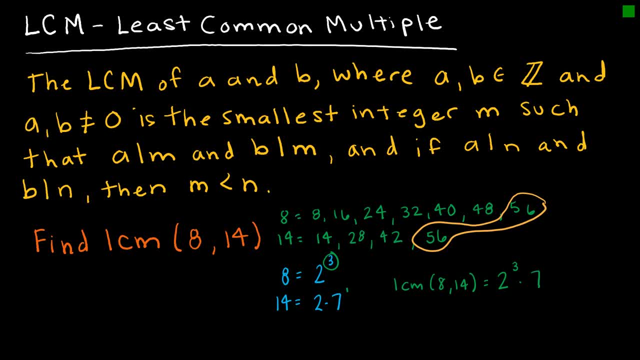 occurs one time, So the most number of times it occurs is once. so 7 to the first. So then I'm just taking 2 to the third times 7, which is 56. So again, this is a strategy for us to use. 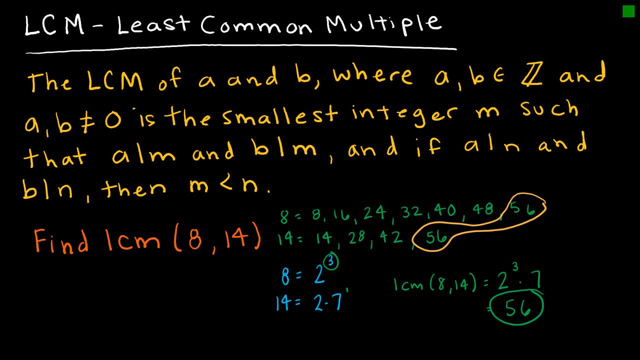 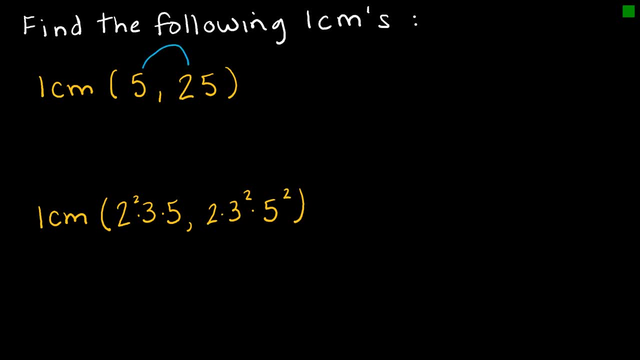 especially if we already have it written as a prime factorization. So again, just a couple of practice, Pretty straightforward. So let's take a look at 8.. 8 is 2 times 2 times 2.. And so again, just a couple of practice, Pretty straightforward. One thing that you can do: 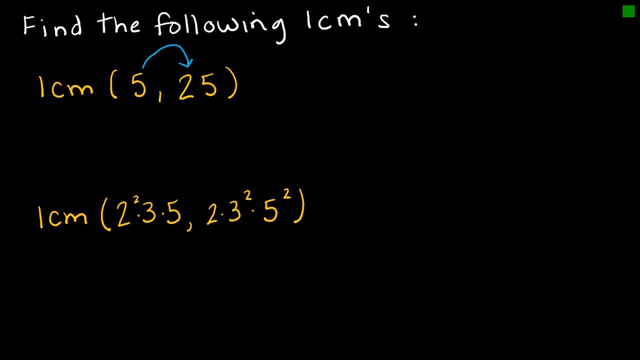 right away- which is why I included this example- is you can say: does 5 go into 25?? Because if it does, there's your LCM right there. You don't have to do any additional work because you know that.